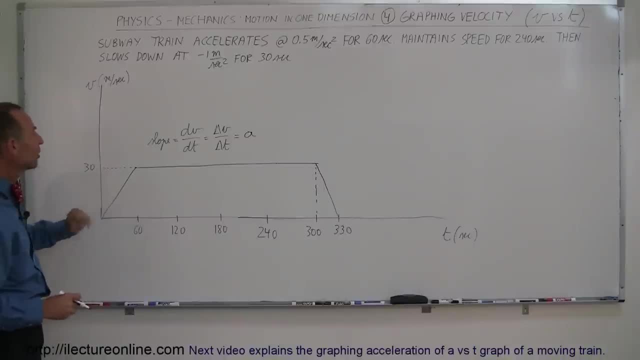 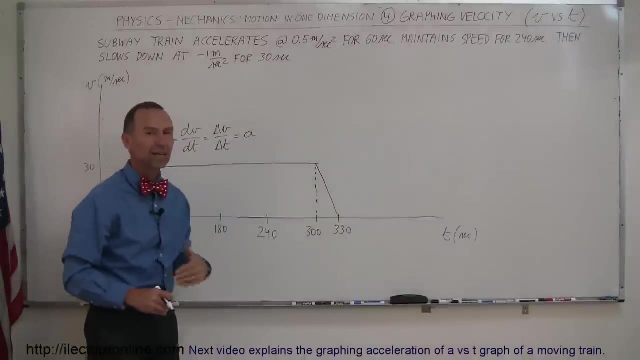 Here the slope is positive. positive acceleration: half a meter per second. squared. Here the slope is 0, 0 acceleration maintains constant speed. Here the slope is negative, it's decelerating or negative acceleration at a minus 1 meter per second. 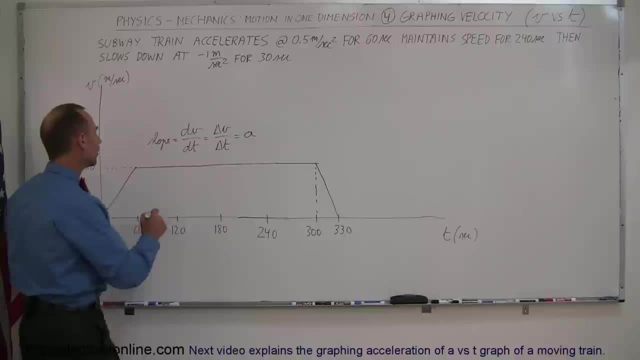 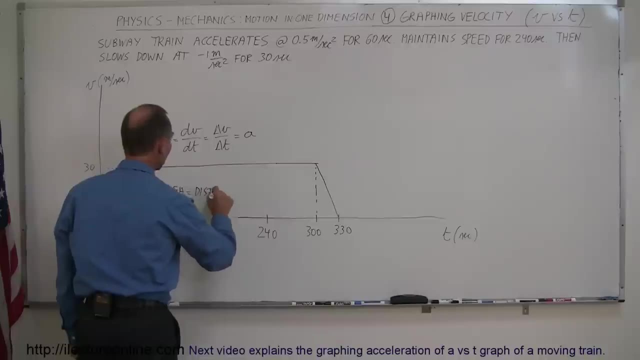 Here the slope is negative. it's decelerating or negative acceleration, at a minus 1 meter per second, squared for the next 30 seconds. What does the area represent? Well, the area represents distance traveled or displacement, if these are vector quantities. 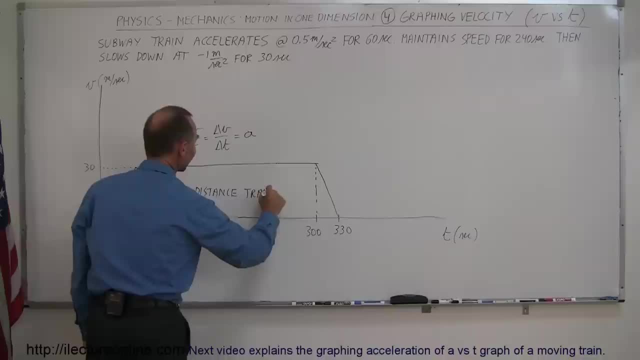 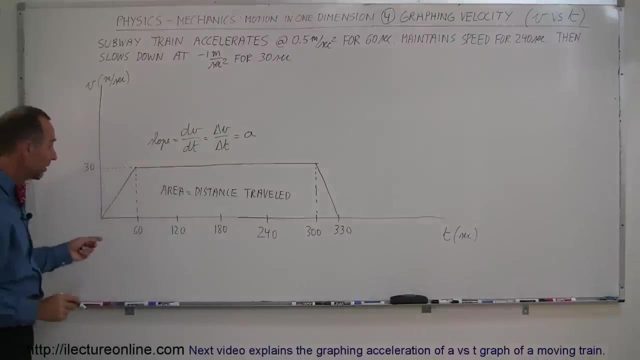 Distance traveled. So let's take a look at this area. Here we have a triangle, So the area of this triangle is one half the base times the height. The base is 60, the height is 30.. 30 times 60 is 1800.. 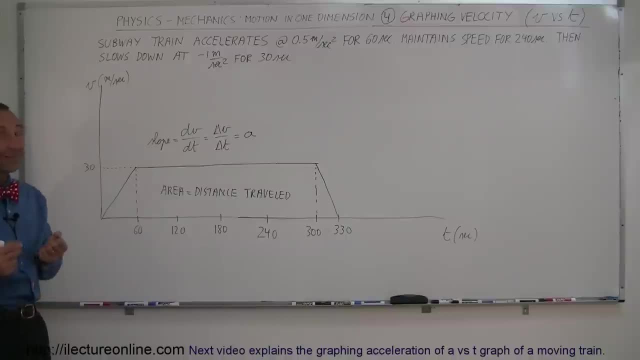 So the area of this triangle is 1 half the base times, the height Times. 1 half, that means 900.. So the train travels 900 meters in the first 60 seconds, Then in the next 240 seconds. how far does it travel? 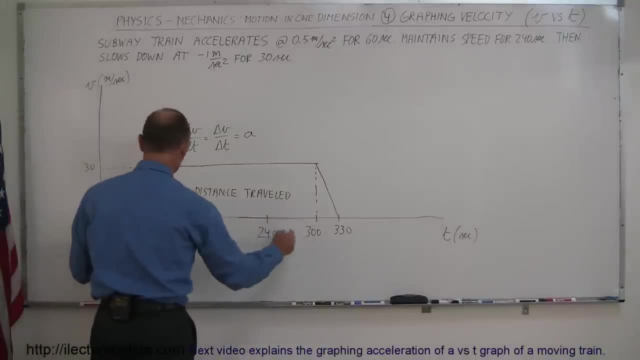 Well, it's a rectangle, so it's height times width, 30 high, 240 wide. So the total there is 7200 meters. And then finally, in this last triangle, it's one half the base times the height. One half the base is 30.. 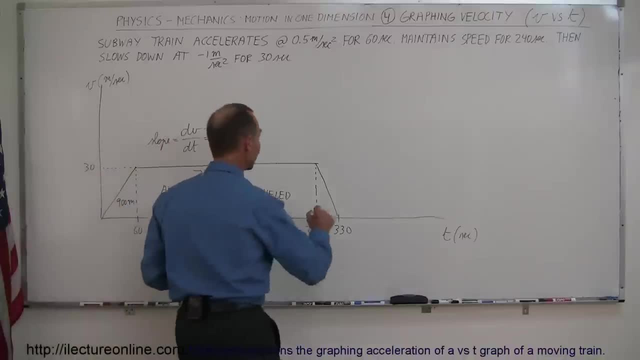 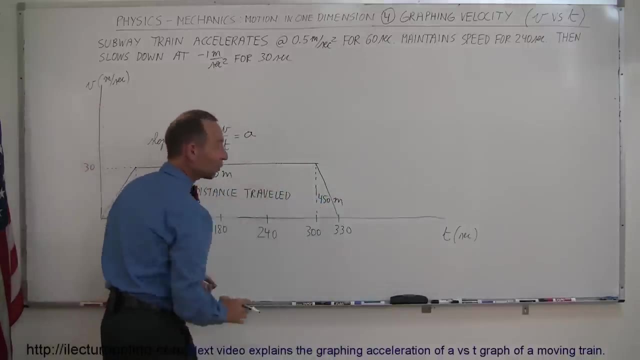 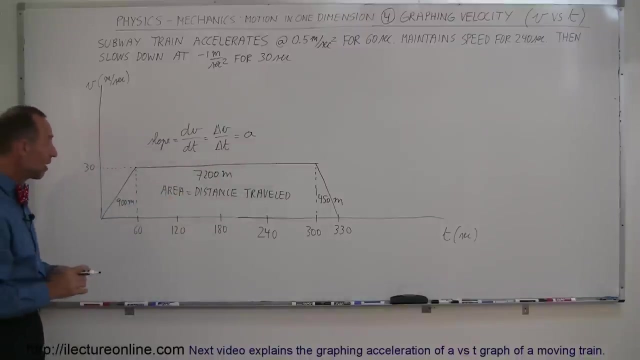 The height is 30.. That's 30 times 30 is 900.. Times 1 half is 450 meters, And so you can see that the total distance traveled is 8100 plus 450, or 8550 meters. So the area underneath the velocity versus time curve represents distance traveled. 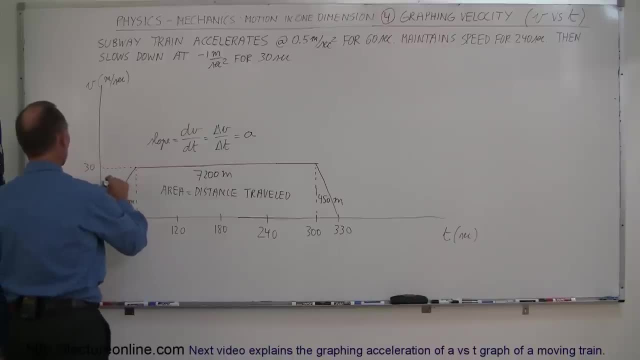 The slope represents acceleration. So here the slope is a positive 0.5.. 0.5 meters per second squared. Here the slope is 0 meters per second squared And here the slope is a minus 1 meter per second squared. 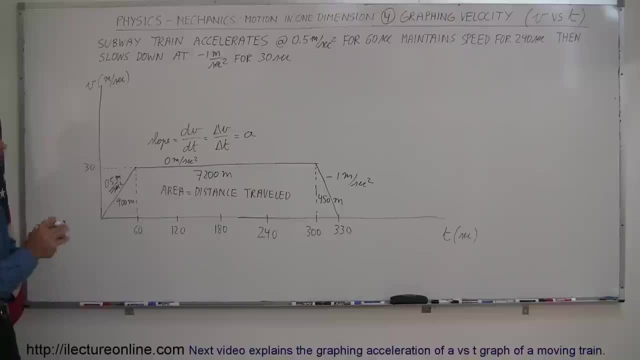 And that's how you draw a velocity versus time graph for an object that starts from rest, accelerates, maintains speed, decelerates, comes back to rest. That's how you do that.